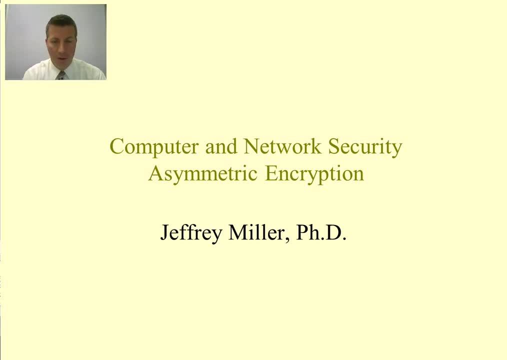 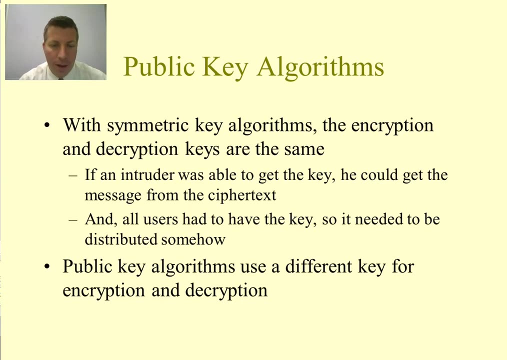 Okay, welcome to Computer and Network Security. Today's lecture is on asymmetric encryption. So, picking up from our last lecture, we talked about symmetric key algorithms, and these are algorithms where the encryption and decryption keys are both the same. So if an intruder 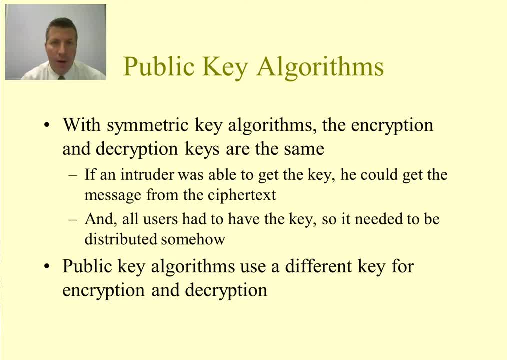 was able to get the key from either of the sender or receiver, they would be able to decrypt the ciphertext and get the plain text back out. In addition, all the users who wanted to be able to communicate on the network had to have the same key, so it needed. 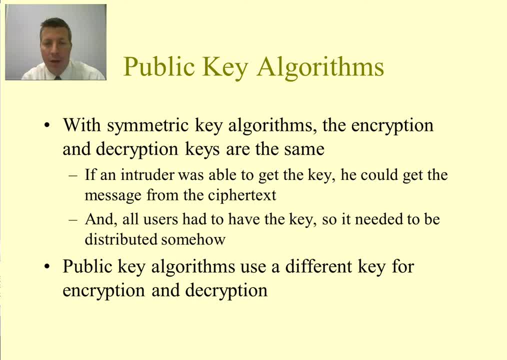 to be distributed somehow, and this was going to be a tough problem of how do we distribute a symmetric key just to the people that we want to have have it, rather than anybody being able to get it. So we are going to talk about how we can distribute keys today. 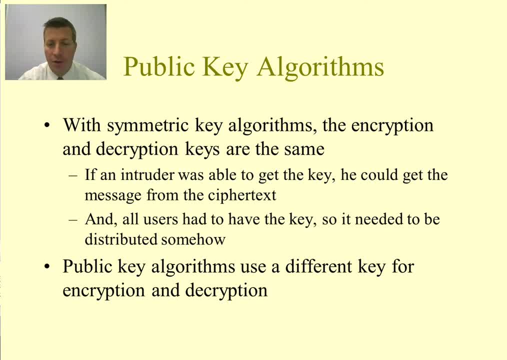 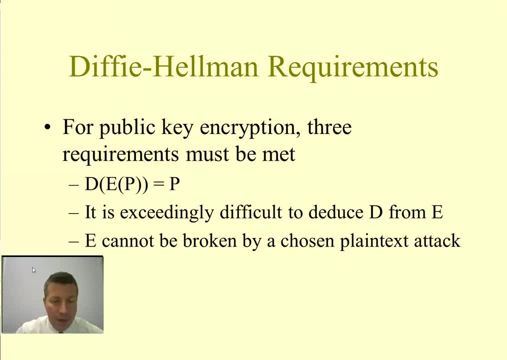 also Public key encryption, which is also known as asymmetric encryption, allows us to use a different key, So the Diffie-Hellman requirements. So two researchers came up with these requirements, So Diffie and Hellman. For public key encryption, we have three requirements that must be met. 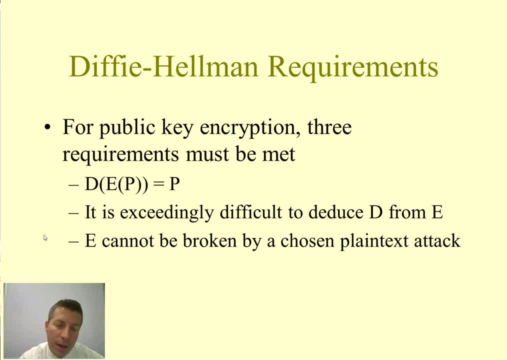 First of all, if we encrypt plain text and then we run that through a decrypt algorithm, obviously we need to get the plain text back out. It needs to be exceedingly difficult to deduce the decryption key from the encryption key. So if we have two keys and then we 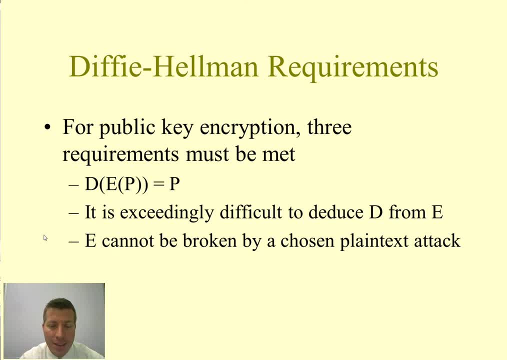 run, one of them gets out. we need to make sure that the other one is not easy to generate and we need to make sure that we can't generate that encryption key. It can't be broken by just any kind of a chosen plain text attack. 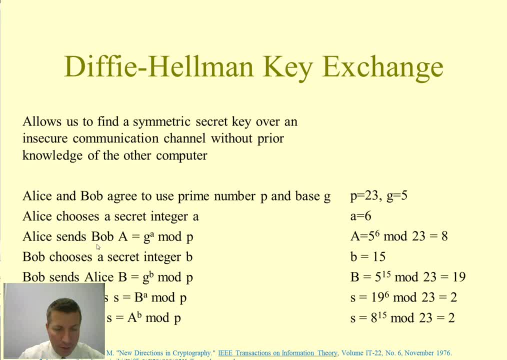 Okay, so Diffie-Hellman also came up with how do we distribute keys, How do we exchange keys? So this was one of the problems that we had in our symmetric key algorithms, and we still have this problem with our symmetric key algorithms. In fact, we still have this. 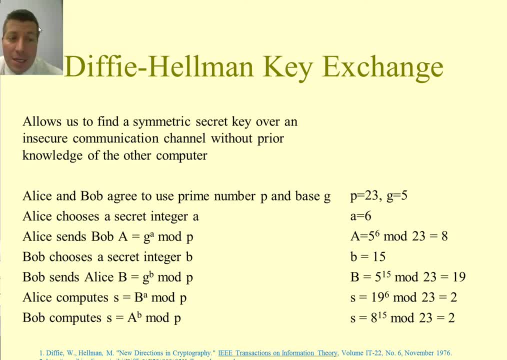 problem with our symmetric key algorithms, which is one of the problems that we had in asymmetric key algorithms- that we need to be able to distribute some keys. So what the Diffie-Hellman key exchange algorithm allows us to do is to find a symmetric secret key over an insecure communication channel. 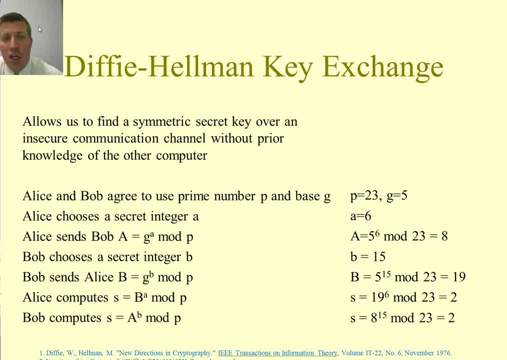 without prior knowledge of the other computer. So how can we exchange these symmetric keys without somebody else in the middle being able to get it? So here is the algorithm for Diffie-Hellman key exchange of symmetric keys. So Alice and Bob want to be able to communicate with each other using a symmetric key. 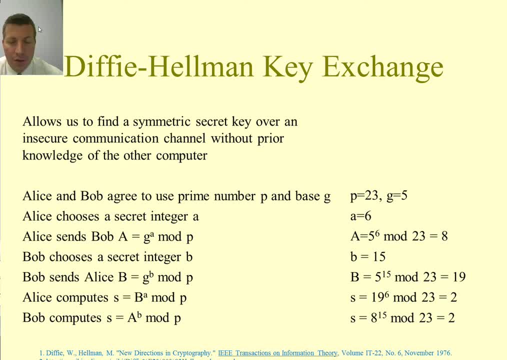 algorithm. So Alice and Bob agree to use prime numbers p. sorry, a prime number p and a base g. These are public numbers, so anybody along the way is going to be able to know these numbers. Both Alice and Bob need to know it, so they had to be able to communicate with each other. 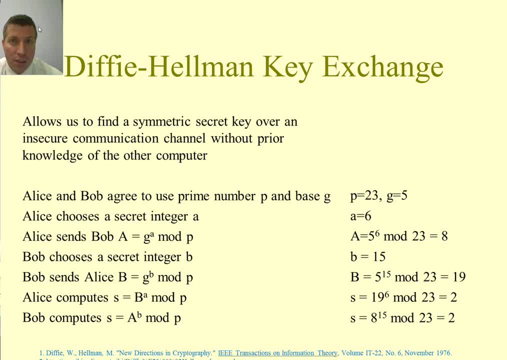 what these numbers were. Alice then chooses a secret, integer a. So Alice keeps this secret. Nobody else is able to get this. Alice sends to Bob a capital A equals g to the a mod p. So a is secret and Alice sends to Bob. 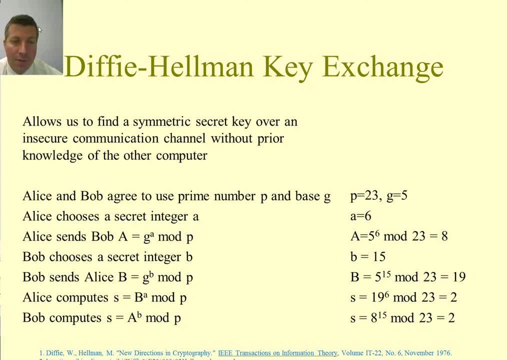 just some number which was generated from the g and the p, which are public, and this secret integer that she's got. a, Bob chooses a secret integer b and he sends to Alice the same thing just the other way around: g to the b mod p and he sends her what comes back from that. 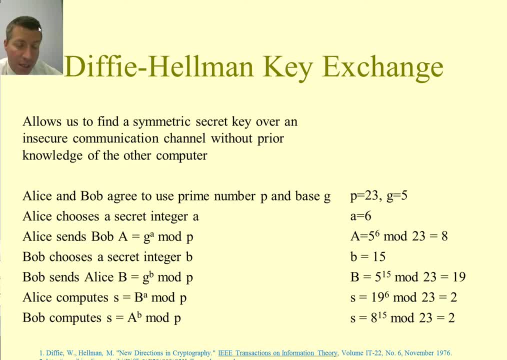 Then Alice and Bob can both compute secret keys s. So Alice computes it with b to the a mod p and Bob computes it with a to the b mod p. So Alice computes it with b to the a mod p and Bob computes it with a to the b mod p. 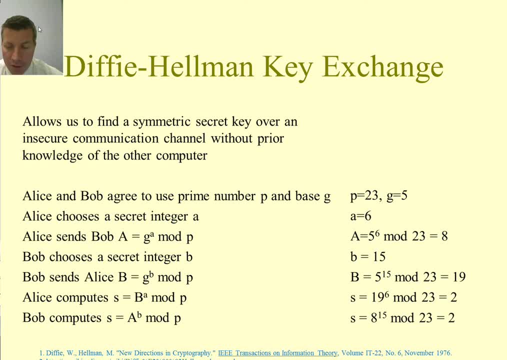 So you can see, using this approach, and you can see the example that I have over here on the right hand side, that what they both did was they both generated the same secret key without knowing, or sorry, the same symmetric key, without knowing what the secret integers were that the other person had. Now these two computers are. 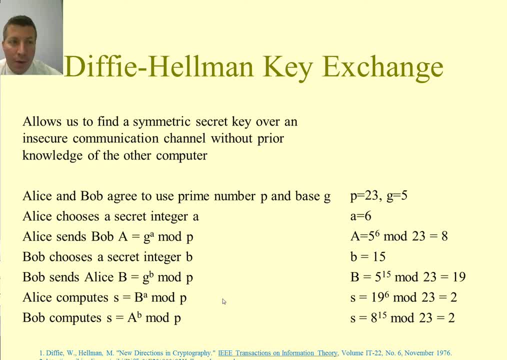 able to communicate with each other without other computers knowing what the symmetric key is. The reason for that is that they generated these keys using their own secret keys and then transmitted that back to the other computer as long as both of those secret integers remain secret. on. 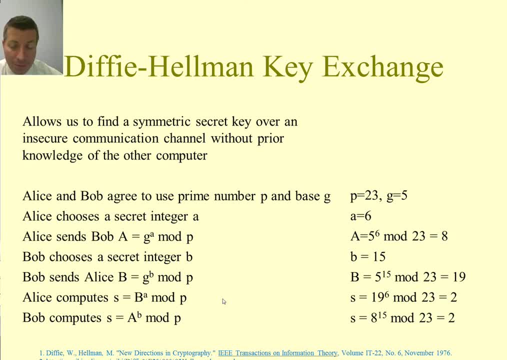 both sides, the symmetric key will not be able to get be retrieved in any real amount of time. Now, of course, there are ways to break any encryption algorithm. brute force is one of the techniques for doing it. However, this little example- here I use very small numbers and you see that it was still a little bit- 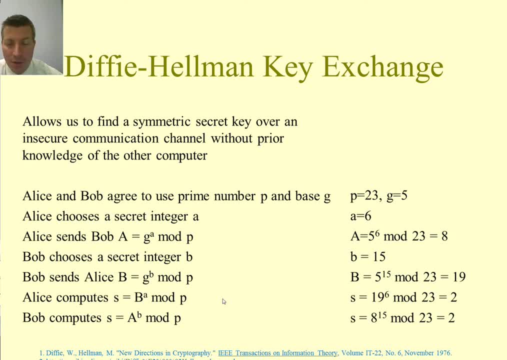 difficult. I mean 5 to the 15 is not a very small number, but when you start using larger numbers, even computers will have a hard time factoring that the product of large numbers or numbers, In this case raising it to exponents. So even those would have a difficult time. 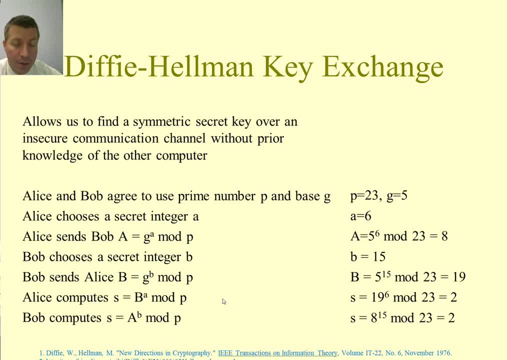 doing it. So this is the Diffie-Hellman algorithm. Look at the paper down at the bottom and new directions in cryptography is the title of that paper. Take a look at that. It's one of the other instrumental papers for encryption. 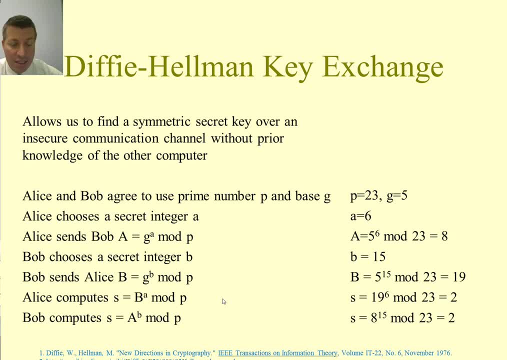 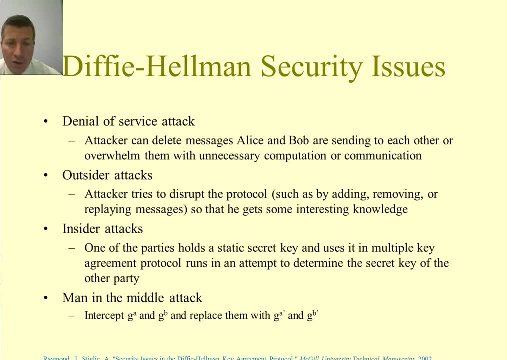 So it was published back in 1976 and it's still quite popular, So go ahead and take a look at that one when you have a chance. There are a few security issues that we have with the Diffie-Hellman algorithm, So when you have a service attack, we're going to have this problem with anything. 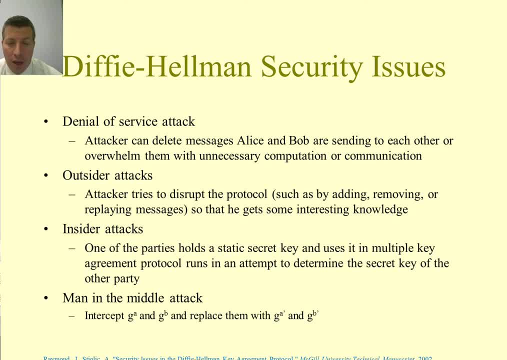 So this is just where an attacker is somehow going to deny service to one or both parties. So here's just an example: an attacker can delete messages that Alice and Bob are sending to each other or overwhelm them with unnecessary computation or communication. Just start sending a whole bunch of messages, That's. 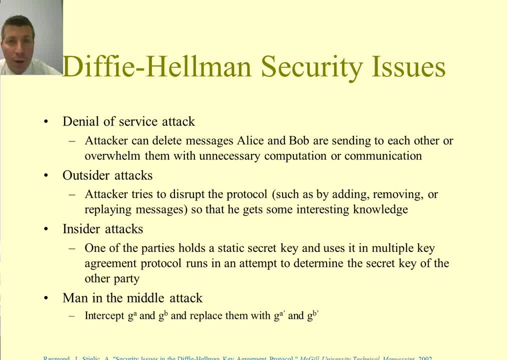 typically how a denial of service attack works is that they, a computer, will become overwhelmed because they're going to be receiving so many messages rather than bad ones, necessarily Outsider attacks. An attacker tries to deny a service to one or both parties. An attacker tries to disrupt the protocol, such by adding, removing, replaying messages. so you get some interesting knowledge. 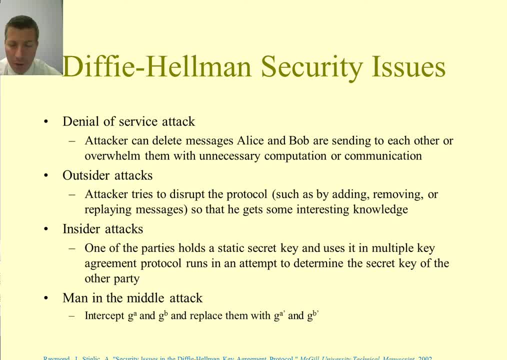 Now, this is an interesting attack, or one of them, where a replay attack is where an attacker actually transmits the same message. it's just that different moments in time to see if they're able to get anything back out of it. So that's an interesting approach. Insider attacks, Obviously, when you have somebody who's 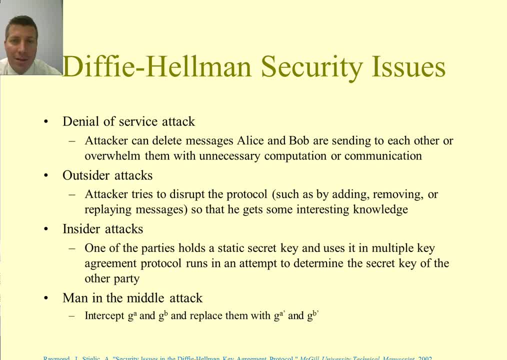 inside of the network they're a little bit more dangerous and cause a little bit more problems than someone who's outside of the network. So an insider attack. One of the parties holds a static secret. He in multiple key agreement protocol runs in an attempt to determine the secret. 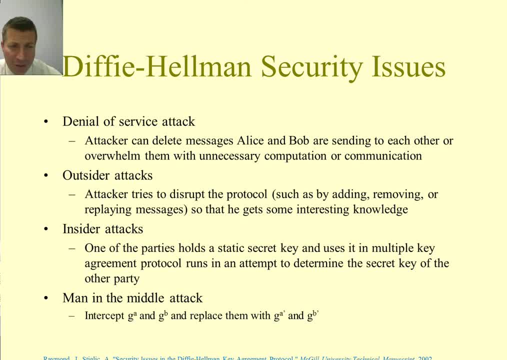 key of the other party. So if you're able to- you know, start transmitting keys back and forth or transmitting messages back and forth, you might be able to find out something about the other messages that are coming back to you. And then, last one, the man-in-the-middle attack. This one is where, when they're transmitting their 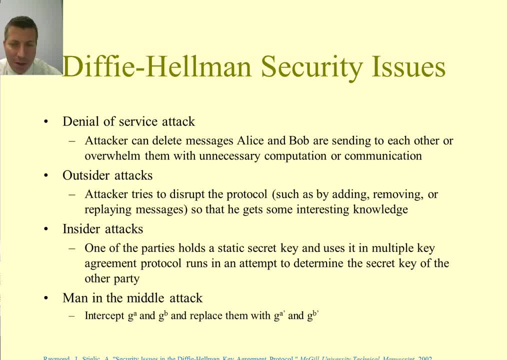 their secret, not their secret integers, but when they're transmitting those public variables back and forth to each other, the values back and forth, the messages back and forth- if somebody's sitting in the middle they can maybe take those and then change them and send them to the other side. And now what they? 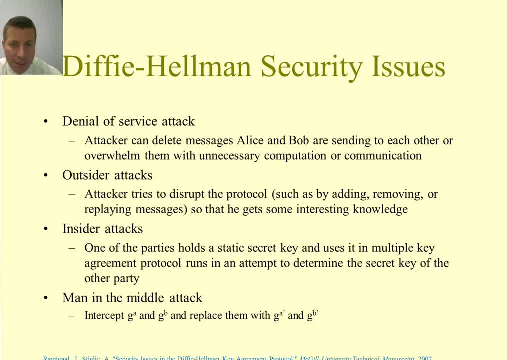 do is they send it back, acting as if they're Bob, if it was Alice sending it to them And Alice thinks that she's actually communicating with Bob, when in fact she's communicating with somebody in the middle And that person is sending a different message with the same data off to Bob and getting the data back. So 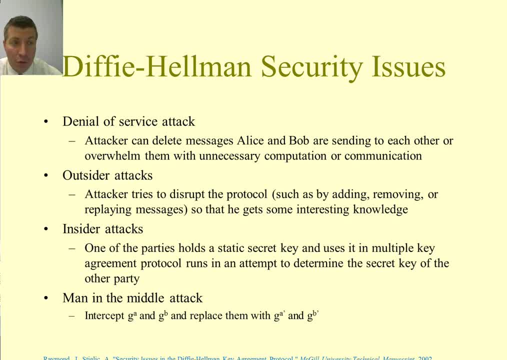 there's nothing that looks fishy to Alice or Bob, because they're getting the messages. They're actually getting them from what seems to be from the other side. So where this is tricky, though, is that they are actually getting it encrypted with a different key than what they think they're getting it with. So that's an. 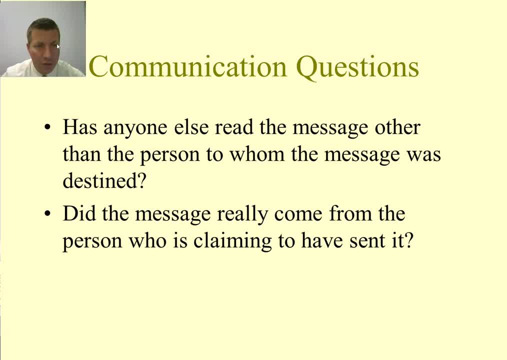 interesting approach there. There's two questions that we want to answer when it comes to communication. The first one: has anyone else read the message other than the person to whom the message was destined to end? The second one: did the message really come from the person who is claiming to have sent it? These are the 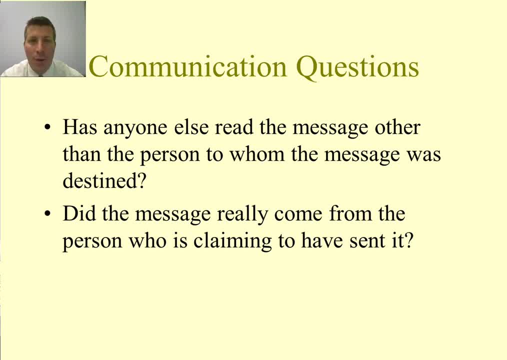 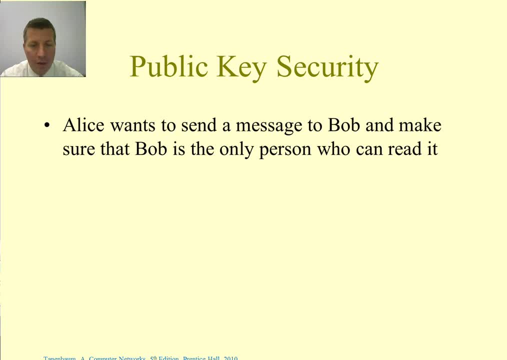 two messages that we have that we want to be able to answer when we receive a message using these encryption algorithms. So here is how public key encryption works. Let's say that Alice wants to send a message to Bob. Make sure that Bob is the only person. 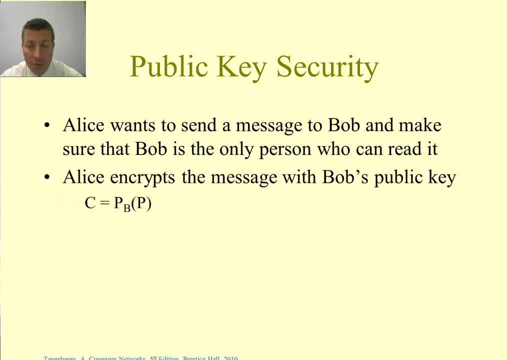 who can read it. So Alice is going to start off encrypting the message with Bob's public key- The public key when we have it. with public key algorithms, we have two keys: We have a secret key and we have a public key. The public key is: 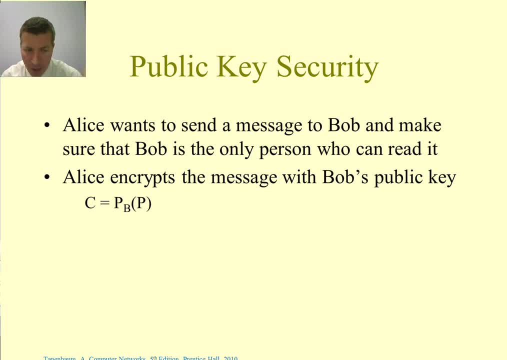 public. Everybody's got access to the public key, So everyone has Bob's public key. If Alice wants to make sure that Bob is the only person who can read it, if she encrypts the message, her plain text, with Bob's public key to produce the cipher text, the only key that's going to be. 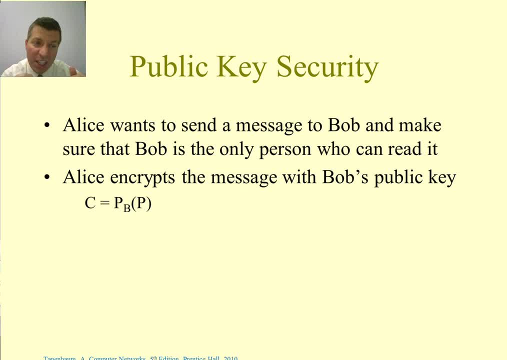 able to decrypt that message is going to be Bob's secret key. As long as he keeps that secret key secret, then he's not going to have any problem because nobody else is going to be able to read that message. So Alice encrypts the message with Bob's public key. Since we have P as the 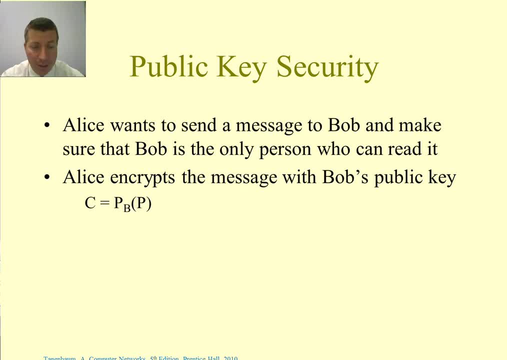 plain text. we'll have P for the public key. We will use S as the secret key instead of using P as a private key. We have a lot of P's coming with this, so we're going to use S as the secret key When Bob wants to decrypt the message he. 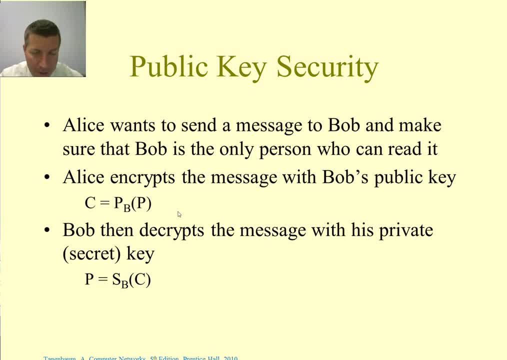 decrypts it with his secret key. So you see that Alice is encrypting the plain text with Bob's public key. This is Bob, so public P, Bob's key B, and it produces the ciphertext. The ciphertext can then be decrypted using: 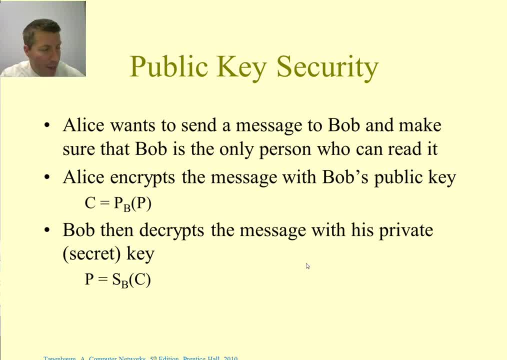 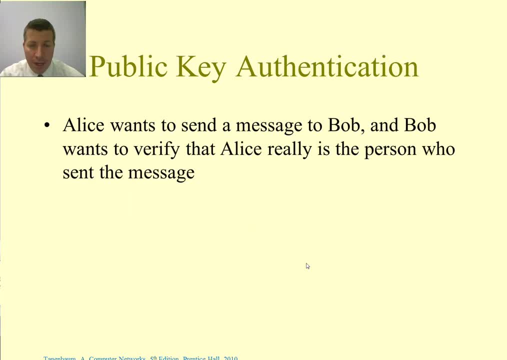 Bob's secret key to produce the plain text back out. Okay, so that's how we can make sure that when we send data to someone, that that is the only person who's able to read it. Now let's look at the next one: the authentication. Now, 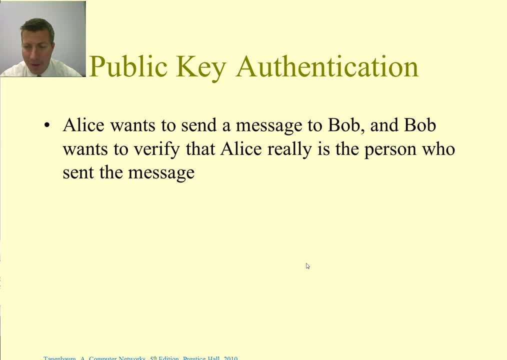 Alice wants to send a message to Bob. Bob wants to verify that Alice really is the person who sent the message. So we don't necessarily care in this case if other people are able to read the message. What we care about here is that we want to. 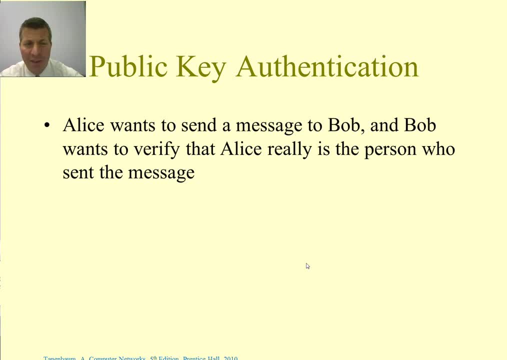 make sure Alice is really the person who sent the message, so that we don't have this problem with this man-in-the-middle attack. So the way that we can verify that is that when Alice sends the message, she's going to encrypt the plain text with her secret key. 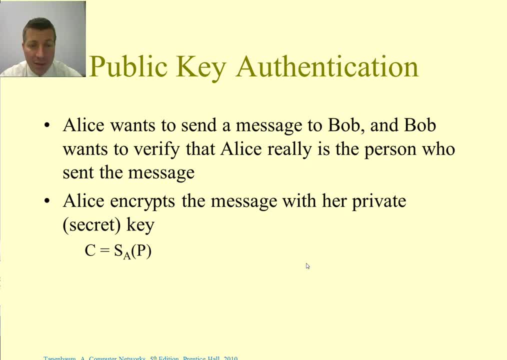 Now, how do we decrypt ciphertext that's been decrypted with a secret key? We use the public key, So Bob is going to decrypt it with Alice's public key. Now, Alice's public key is public and everybody has access to her public key, but that's okay, because we're not so interested in making sure that no one is. 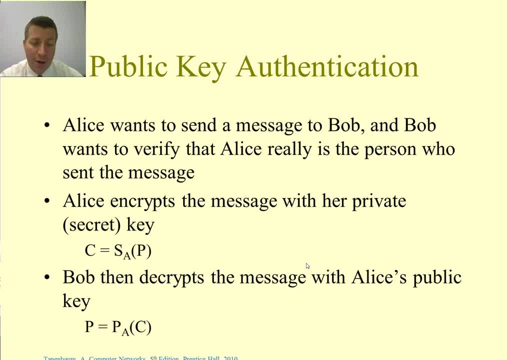 able to read the message that Alice is sending. Instead, we just want to make sure that we can verify that Alice really is the person who sent the message, And we can do that. if Alice encrypts it with her secret key, then we can decrypt it with her public key. 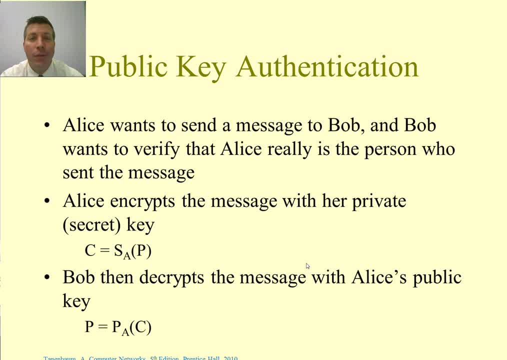 And that way, if we were able to decrypt it, we know that Alice really is the person who sent it. And this is all, of course, assuming that the secret key has remained secret. If that got out, then we're not going to be able to say anything. 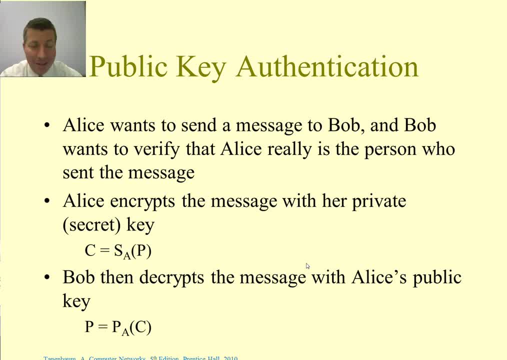 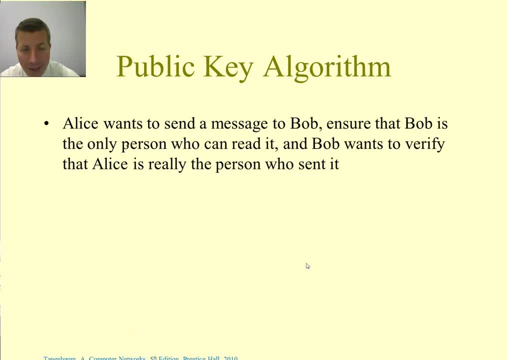 about it, But we're probably not going to know that either. So as long as the secret key remains secret, we will be able to verify that Alice really is the person who sent it. Now what if we want to do both? Alice wants to send a message to Bob to make sure that. 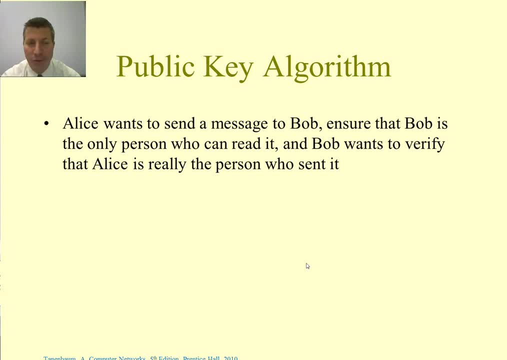 Bob is the only person who can read it, and Bob wants to verify that Alice really is the person who sent it. so what we're going to do here is we're just going to encrypt twice, okay. so what we're going to do here is we're just going to do. 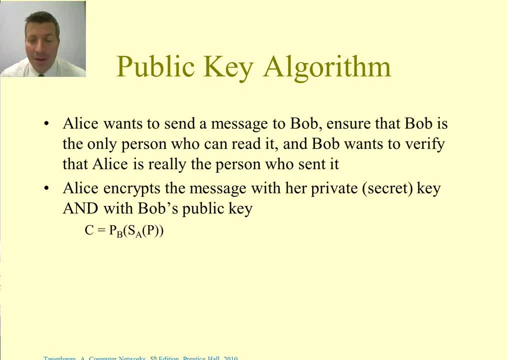 both of them we're going to. first of all, Alice is going to encrypt the message with her private key or secret key, and then that ciphertext she's going to encrypt with Bob's public key. now, what that means encrypting in this order is that you're gonna have to first decrypt with Bob's secret key and then after you. 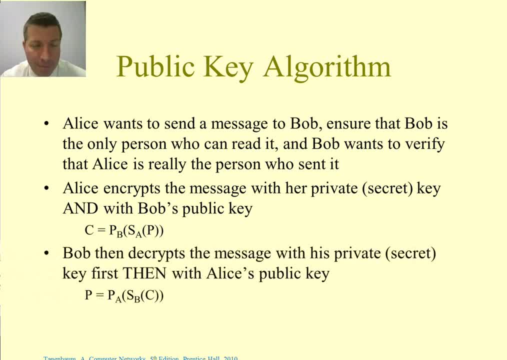 decrypt the Bob's secret key, you're gonna have to decrypt with Alice's public key. so we do it in the reverse order when we're decrypting as opposed to when we're encrypting. now we probably want to do it in this order, where instead some people may be tempted to say, well, let's encrypt the plaintext. 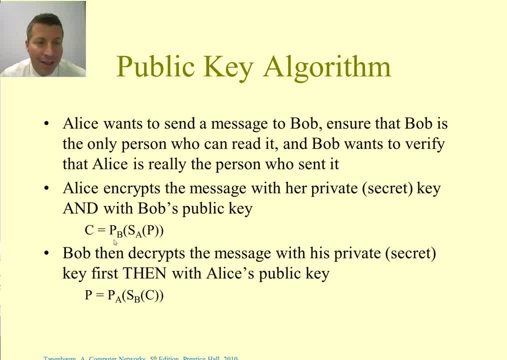 with Bob's public key and then encrypt that with Alice's secret key. the only problem with that is that you've gotten rid of that second part of the algorithm, then, because everybody has Alice's public key, so anyone would be able to decrypt it with Alice's public key, and then they would just have one more thing. 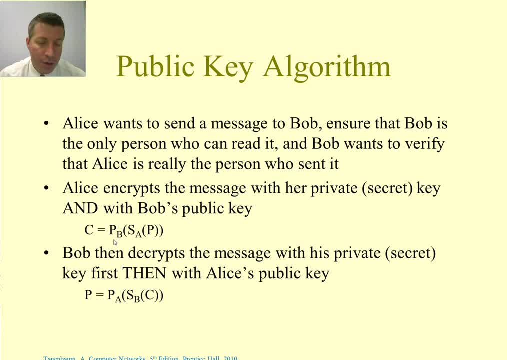 to crack to be able to get the, and then they would just have one more thing to crack to be able to get the plain text back out. When you do it in this order, the first thing that you have to do is going to be decrypted with Bob's secret key, which nobody should have other than Bob. So this is probably 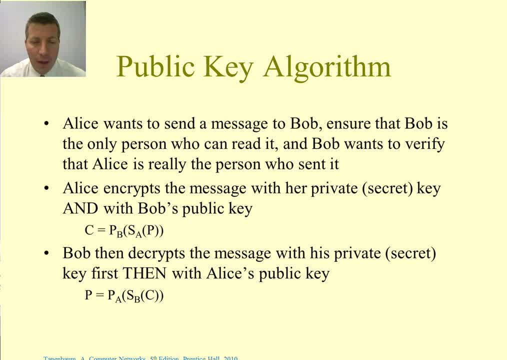 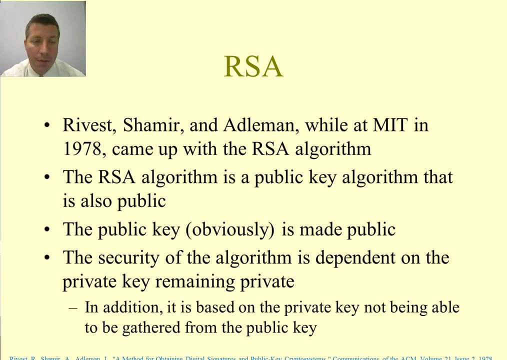 a little bit more secure way of making sure that Bob is the only person who can read the message and that Alice really is the person who sent the message. Okay, one of the most popular public key algorithms in existence is RSA. RSA actually stands for the name of three researchers who 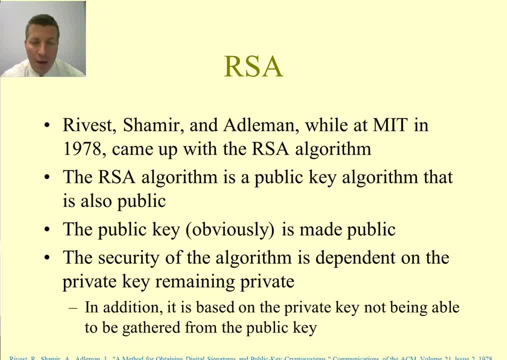 created it. So this is Rivis Shamir and Edelman, And while at MIT in 1978, they came up with the RSA algorithm. It's a public key algorithm and it also is public. The public key is made public. 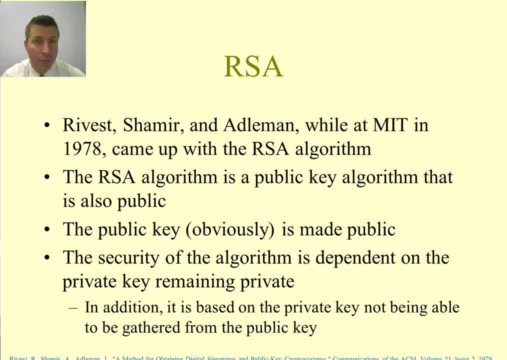 to everyone and the security algorithm is dependent on, obviously, the private key remaining private. As long as that's the case, then this algorithm is going to be rather secure. It has been in existence now for a long time- 30,, what 30? some years or so. 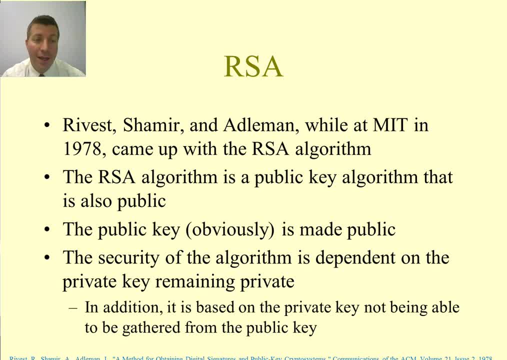 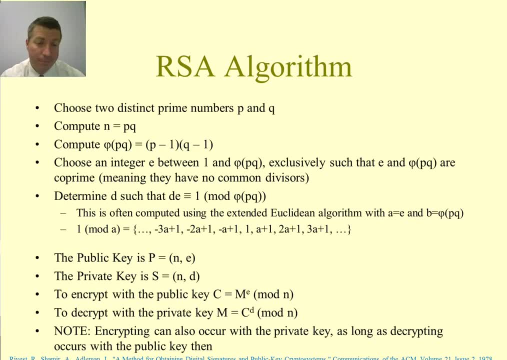 And no one has been able to crack the algorithm, and I'll show you exactly what it is because it abides by Kirchhoff's principles of being public. So here is the RSA algorithm. So you start off by choosing two distinct prime numbers, P and Q. You compute: N equals P times Q and you compute. 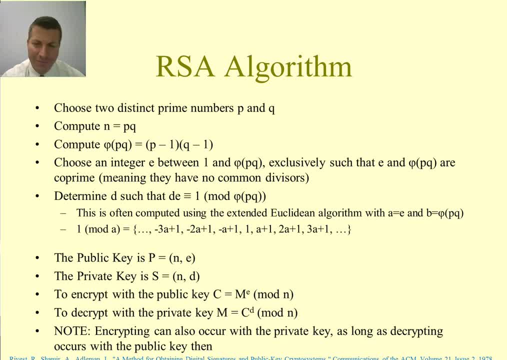 phi of PQ is P minus 1 times Q minus 1.. Relatively easy so far, Generating the prime numbers. that might be a little difficult, especially because you probably want to generate very large prime numbers If you generate small prime numbers, the example I'm going to give you today. 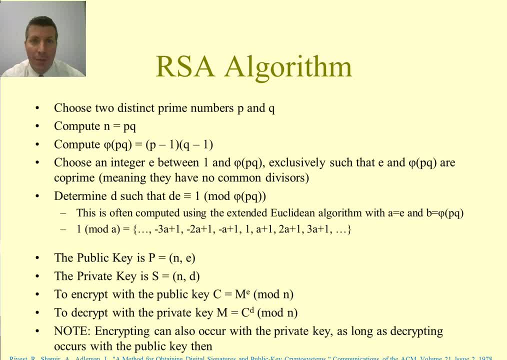 we use very, very small prime numbers, because otherwise it's going to make it very hard for us as humans to calculate some of the things that we need to. Okay, step four: choose an integer E which is between 1 and 5 PQ exclusively, such that E and 5 PQ are co-prime. That means that they have 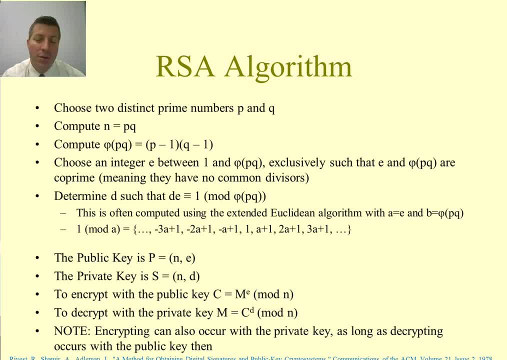 no common divisors. So between those two numbers, the only numbers that are going to divide them evenly will be 1.. No other number will divide the two numbers evenly. So that's what it means if those two numbers are going to be co-prime. 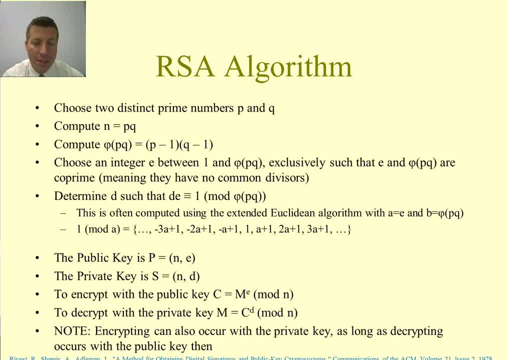 And then the last step, determine D such that D times E is in the set of 1 mod 5 PQ And 1 mod 5 PQ. so I gave a little example here of what does it mean if 1 mod A. This is actually a set of numbers. 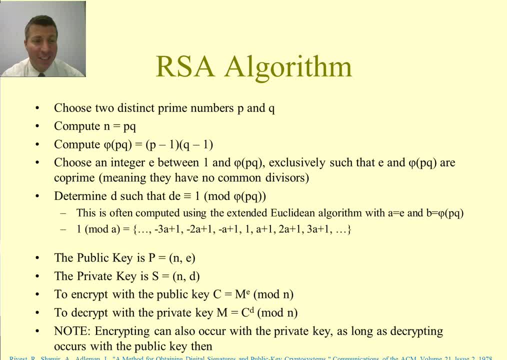 Now you probably have learned the mod in the percent sign in some of your programming classes and you learned that the result is always going to be between 0 and in this case here, if it was 1 mod A, then the answer would always be between 0 and A minus 1.. 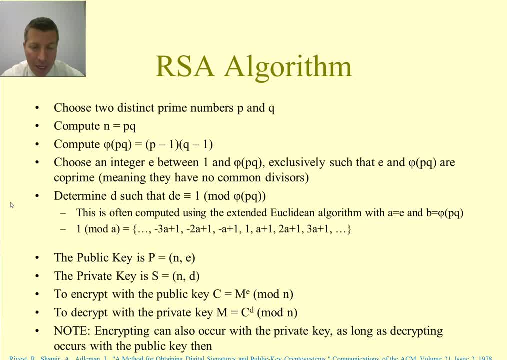 Inclusively. But this is actually going to be a set that comes back, where you can take that number and then you just add A to it. So what I want is: I want to want to know that D times E here that I have on the left-hand side is going to be. if I do a D times E mod 5 PQ, what I want to get is a 1.. 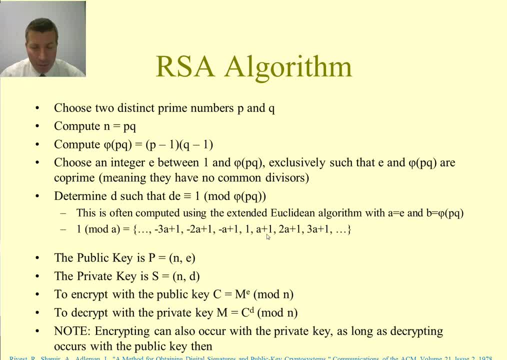 And so there's going to be a lot of numbers that abide by that, such as A plus 1, 2A plus 1, 3A plus 1, and so on, if A is what I have here On the right-hand side inside of my mod equation, So this is a set. 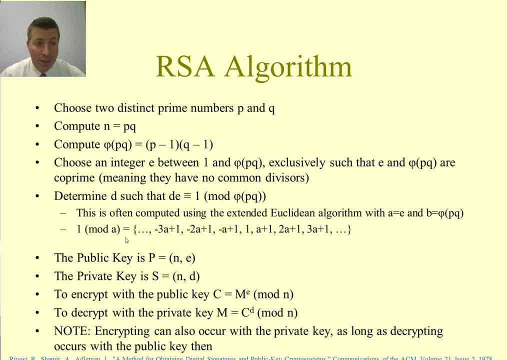 You can look up more information about the mod algorithm, the modulus algorithm, but this is actually a set of numbers, So there are a lot of different numbers that are going to abide by that. What's going to be difficult, though, is, since we already know what our value E is. what's going to be difficult? 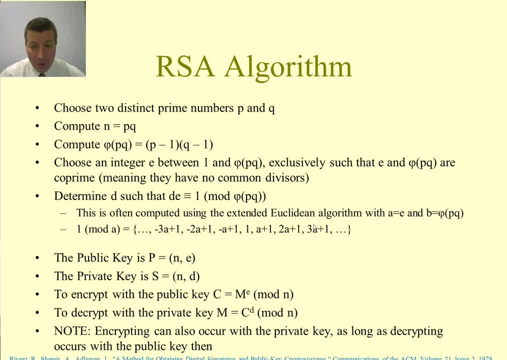 is how do we generate this value D such that this D times E is going to fall somewhere into the set that we're looking at The way that we do that? there is an algorithm called the extended Euclidean algorithm. I'll show you that algorithm here in just a second, And it takes two parameters. 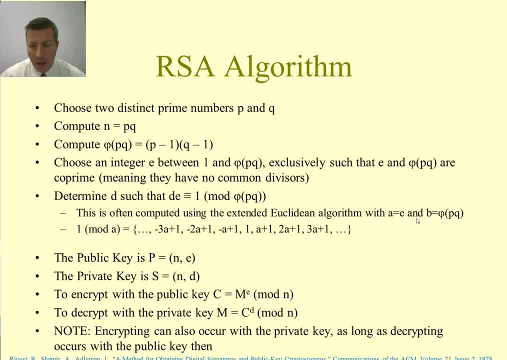 There's an A and a B. So if we use E as our A and phi of P, Q as our B, we're going to be able to solve that and get our value of D Okay. so once we do that, those are the five steps of the RSA algorithm. 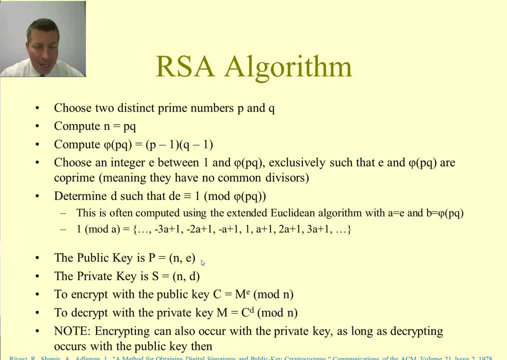 And the public key is then going to be N and E and the private key is N and D. So you just need to keep this variable D that you generate here in this fifth step. You keep that secret and you have your private key for the RSA algorithm. 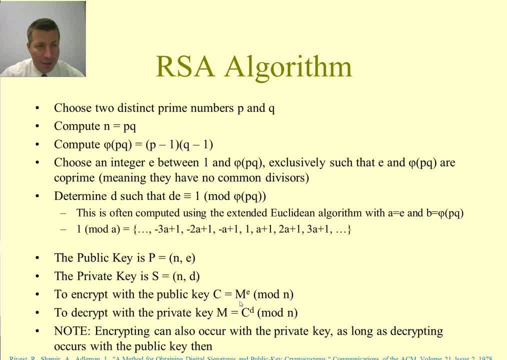 To encrypt it. we use this formula here, So our ciphertext is going to be our message here. This is our plaintext: M Raise that to the E mod N. You're going to have to somehow figure out how you're going to represent your plaintext. 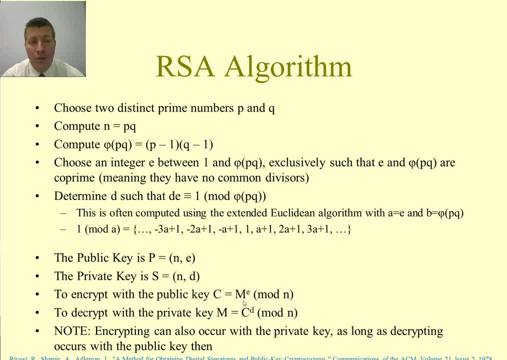 This could just be an ASCII value. Each character can be encrypted individually. You can group them together into some kind of a logical ordering and then raise that to the E power and then modify N and so on. So however you're going to do this, it just has to be agreed upon to the other side. 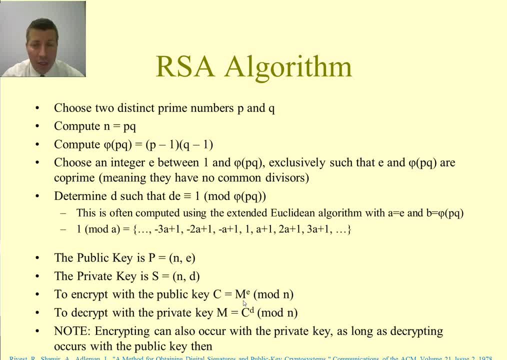 ASCII is typically a good way of doing it. You encrypt each character individually, You could encrypt the entire character individually, You could encrypt the entire file, depending on how you've represented the file, and so on. To decrypt it. then to get your plaintext back out, your message, you're going to take your ciphertext, raise it to the D power. 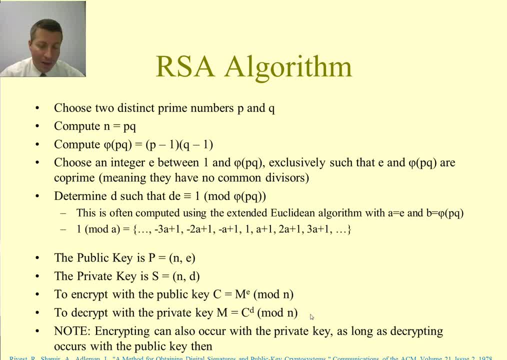 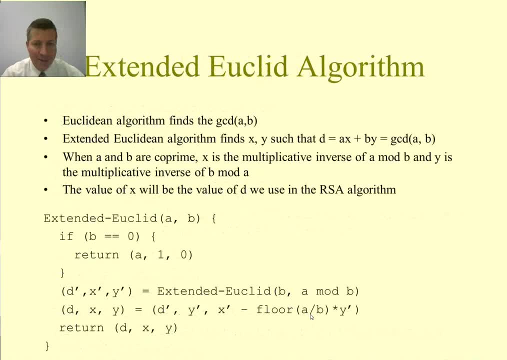 Remember, this is going to be your private key. It has D, And then mod that by N and that will get your plaintext back out from your ciphertext. Okay, so we're going to go through an example. I'm going to show you how the extended Euclid algorithm works. 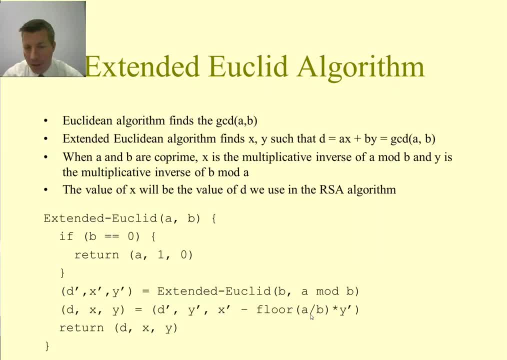 And then we're going to walk through an example using RSA. So the Euclidean algorithm finds the greatest common divisor of A and B. The extended Euclidean algorithm finds X and Y such that D equals AX plus BY, which is the greatest common divisor of A and B. 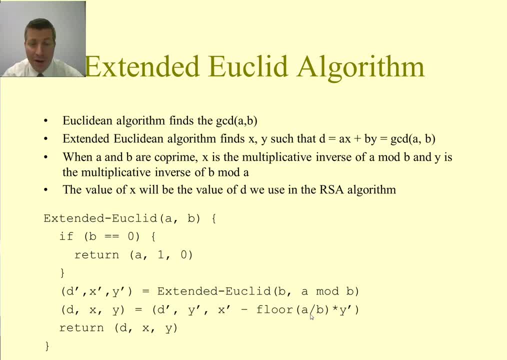 When A and B are co-prime, which is what we know, X is the multiplicative inverse of A mod B. Y is the multiplicative inverse of B mod A. So what we're going to do is we're going to run this algorithm. 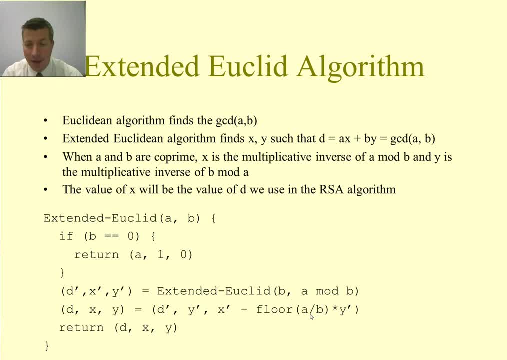 We're going to get the value of X back out And we're going to use E for the value of A And we're going to use 5PQ as the value of B And then our value X. that comes back out. 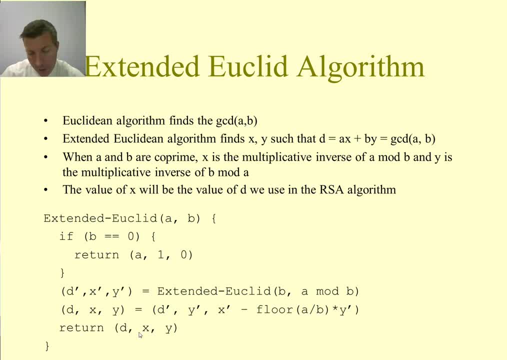 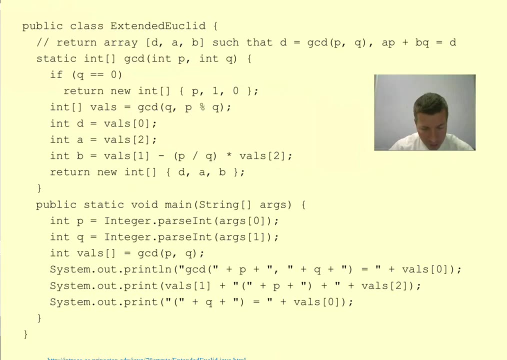 That's returned from our algorithm down here. Our value X is going to be our value D that we need for our RSA algorithm. Okay, I found some Java code for the extended Euclid algorithm here- The website down here at the bottom you can see this. 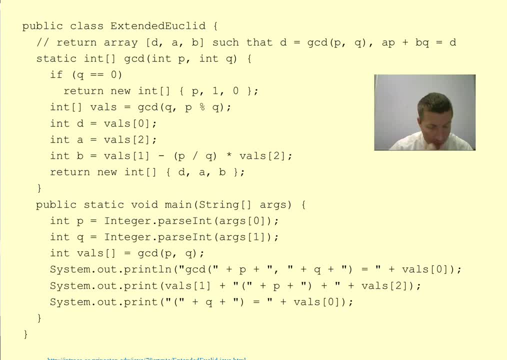 It's from a website at Princeton. It was copywritten Robert Sedgwick and Kevin Wayne. But this algorithm here, this is the extended Euclid algorithm, So you can see the exact code for it. It walks through the algorithm that you just saw on the previous slide. 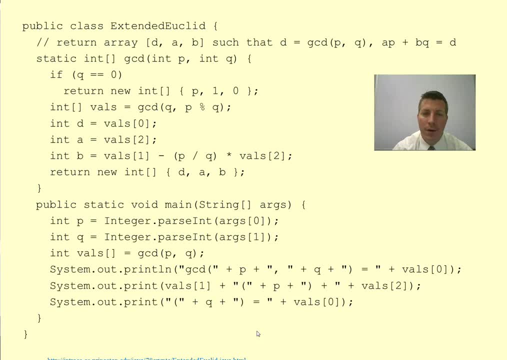 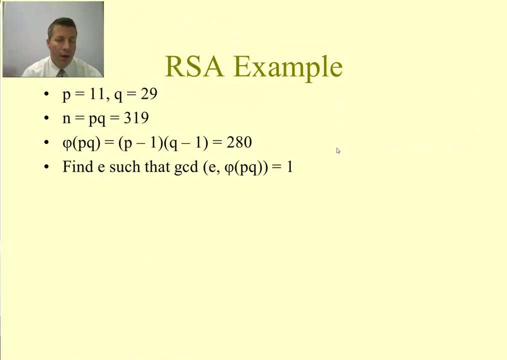 And I'll run this in just a second on our example of RSA, So you can see this run and see the values that are generated from this algorithm. Okay, so here is the example of RSA that we're going to go through. So we start off with two values: P and Q. 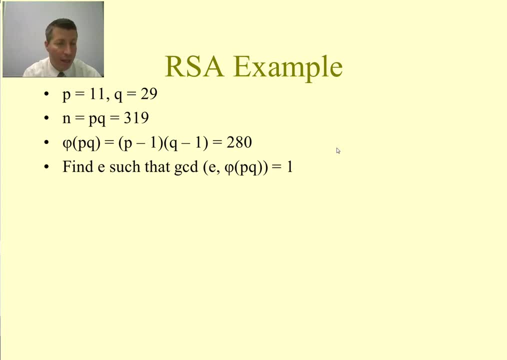 So I chose 11 for P and 29 for Q. They just both needed to be prime numbers. That was our first step. Our second step, compute N of which is the product of P and Q. So N equals PQ is 319. 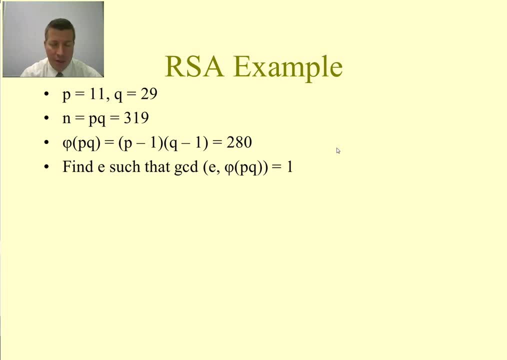 5PQ. the product of one less than each one of those is 280.. Now we get to a little bit more difficult part. We need to find E such that the greatest common divisor of E and 5PQ is equal to 1.. 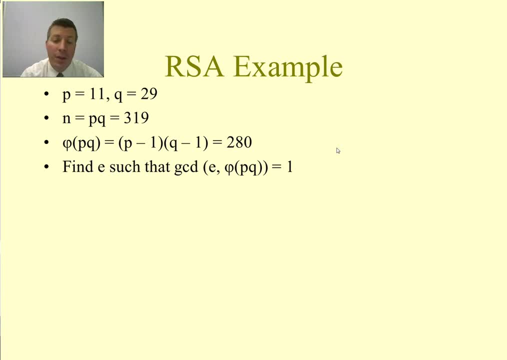 So we just need to find some value of E such that there are no common divisors between E and 5PQ other than 1.. One easy way that we can do this Is a prime number. So you see here that I've taken 3 as my value of E. 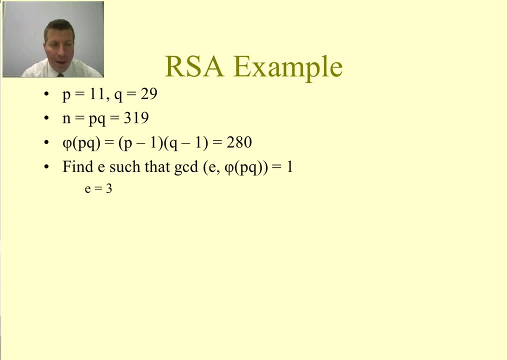 3 does not divide 280 evenly And there are no other divisors of number 3. So that means that this number is going to be relatively prime to 280 to 5PQ. Now here comes the step where we need to use the extended Euclid algorithm to find D such that DE is in the set of 1 mod 5 of PQ. 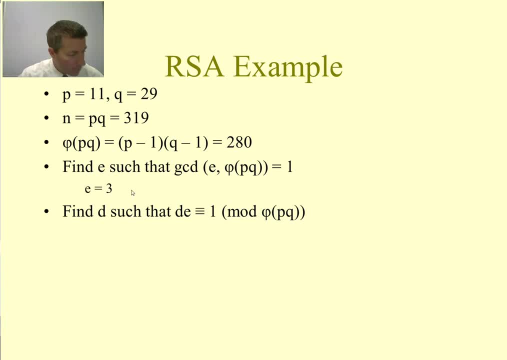 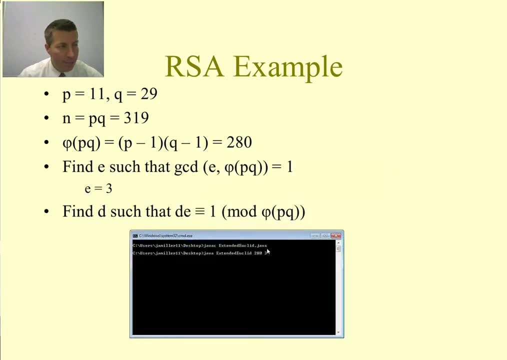 So 5PQ is 280. E is 280. E is 3.. So if we run our algorithm now, The extended Euclid algorithm. So I compiled the extended Euclidjava file that I showed you on the previous slide. 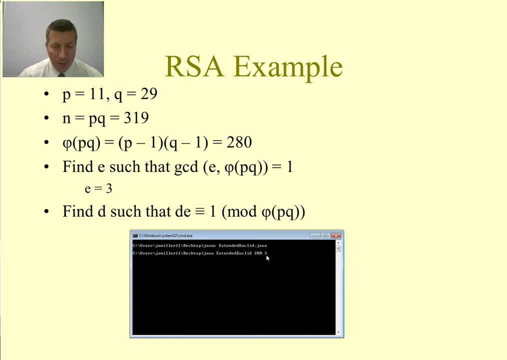 If we run this now with 280 as our A and 3 as our B. So remember we're going to use 5PQ and E as our two values. You can actually switch these around because if you notice from the algorithm, Let me show you that again here. 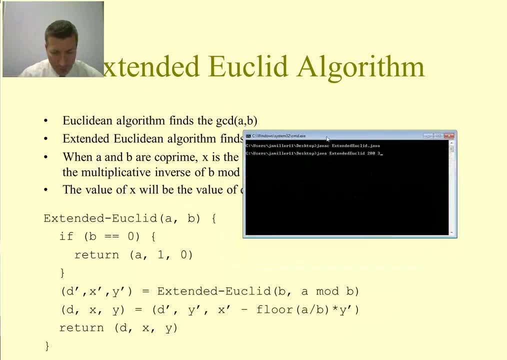 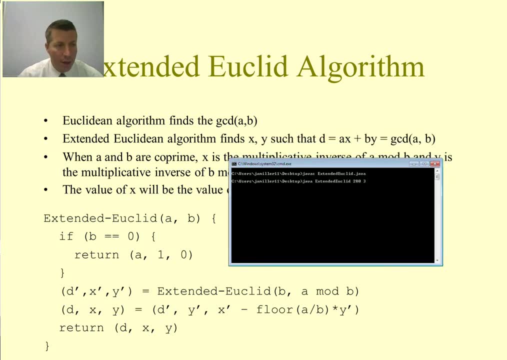 If you notice from the algorithm What it does here is it switches them around right off the bat here. So if you happen to reverse them, It's going to switch them around. It's still going to work out just fine for you, Okay. 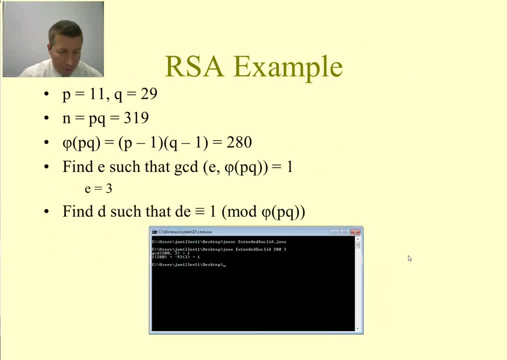 So let me go ahead and run this algorithm here, And you see that what pops out here is going to be this: 1 times 280 plus a negative 93 times 3 equals 1.. The number that we want is that one, right there? 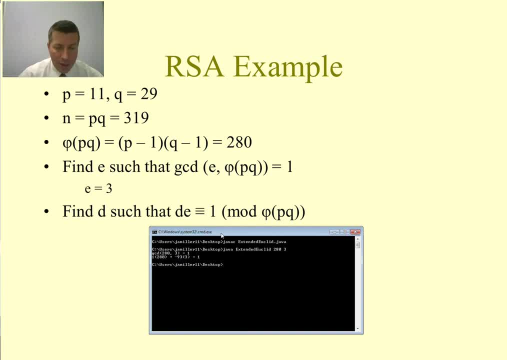 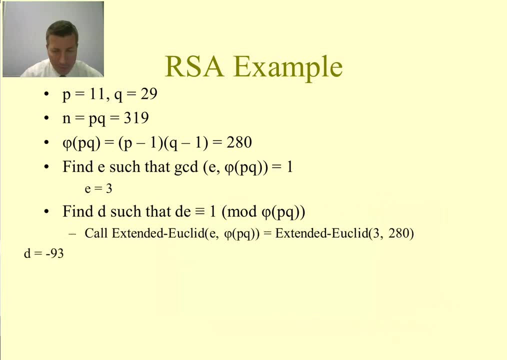 That negative 93.. So negative 93 is going to be our value of D. Okay, So there's our public key and our secret key If we want to verify this negative 93. Let me go ahead and pull up a calculator here. 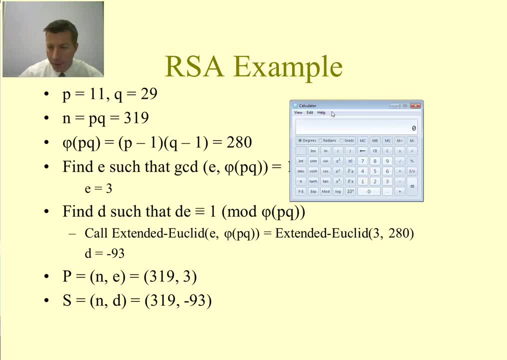 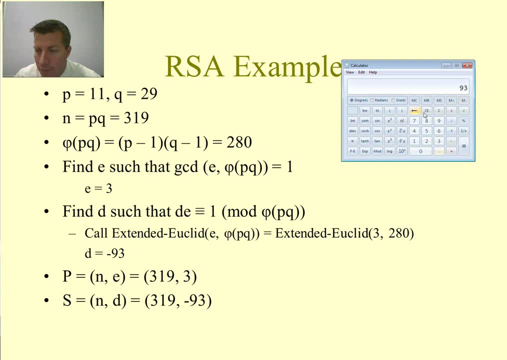 And show you that that number is correct, So you're not just believing that algorithm there. So, if I take 93.. Okay, There's my negative 93 now And I am going to- Okay, I'm going to multiply that by 3.. 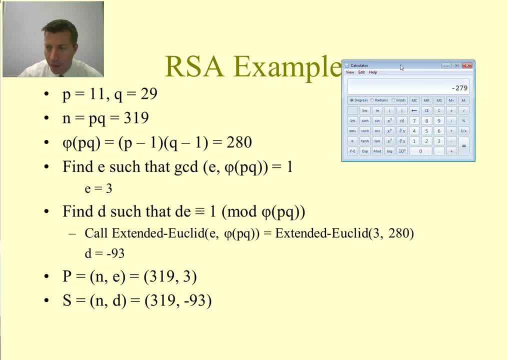 Because that's that D times E that I have right there. So I'm going to multiply this by 3.. That gives me negative 279.. And you see that negative 279 compared to 280 is going to have a remainder of 1..